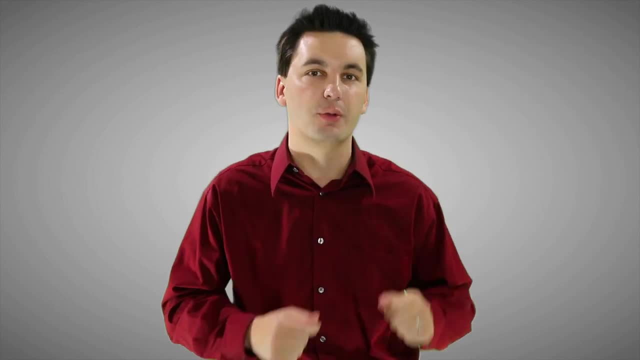 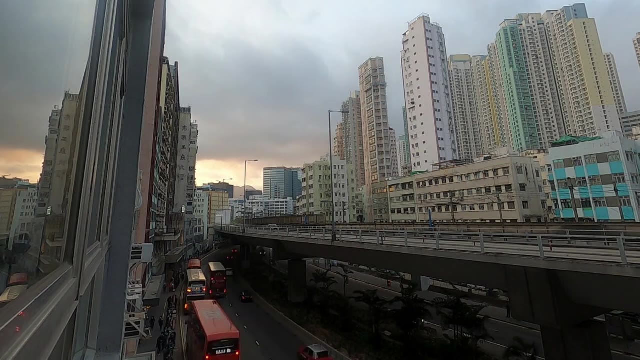 going to be important to understand that, because this topic builds off the previous standard. As countries and cities and regions change and their populations fluctuate, we can see that we have political, economic, social and environmental factors and challenges that they're going to have. 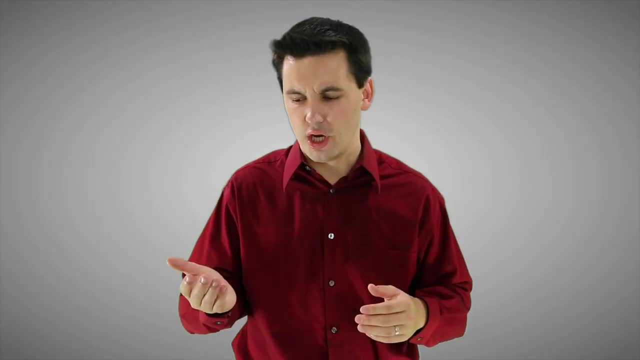 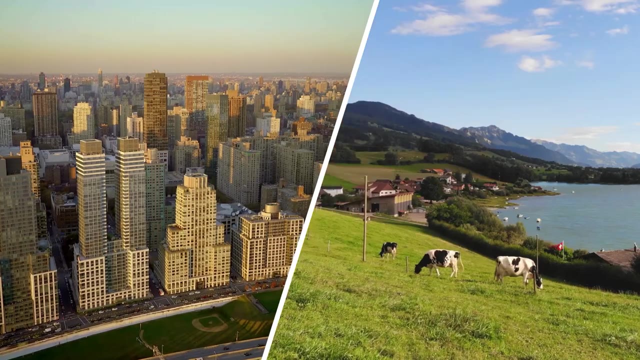 to deal with Politically. we could look at how, as society grows and changes and evolves, our population distribution becomes more uneven, More and more people start living in urban areas and less people live in rural communities, And what starts to happen then is that sways. 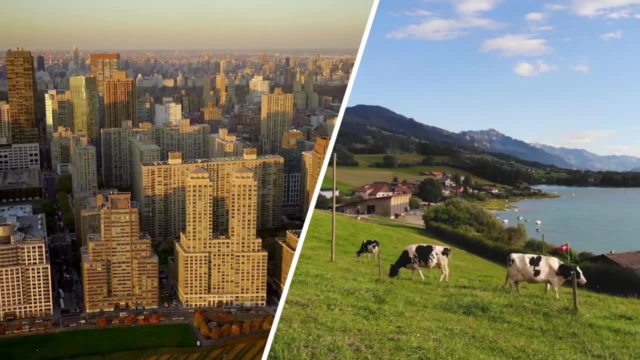 the political power towards larger cities, as they have more people who are voting on matters, and so politicians give them more time and also focus on their needs more. On the other hand, there's a lot of people who live in rural areas, and they don't have 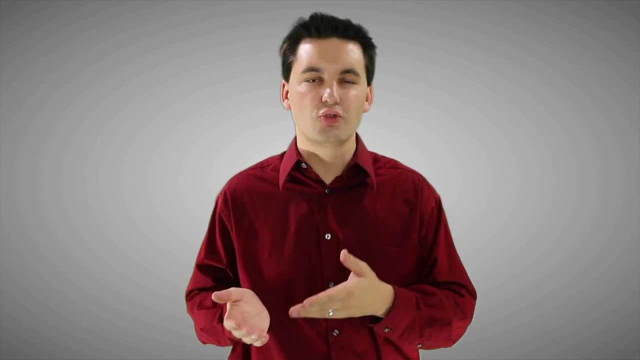 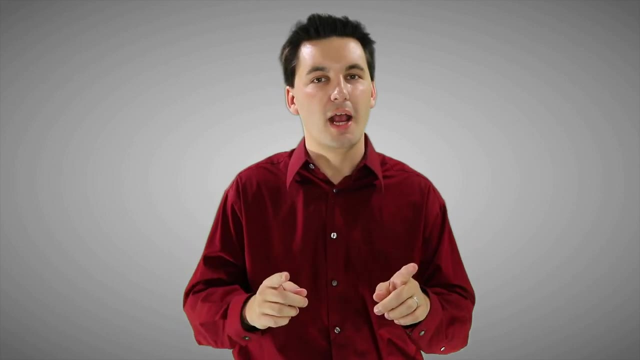 enough money to live in rural areas. On the other hand, though, we could also look at how the political power of an individual actually diminishes if they're living in a large urban area or if they're living in a state with a big population, compared to the political power of 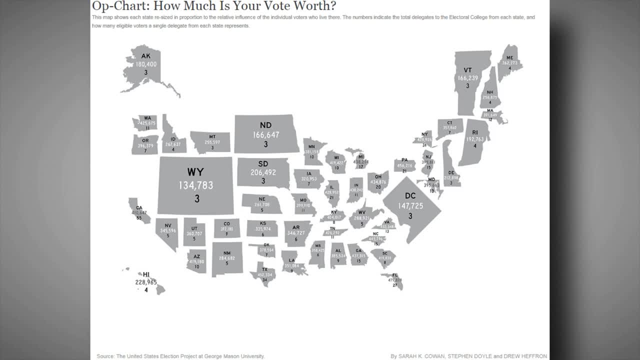 individuals in smaller states or smaller communities. For example, in the United States, citizens who live in a state with less people living in it actually have more impact on where the electoral votes for their state will end up going, compared to citizens who live in a larger. 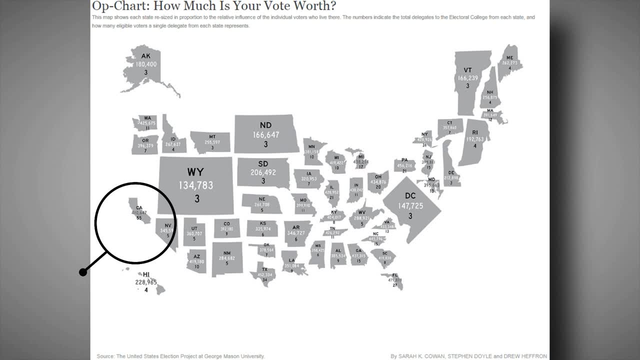 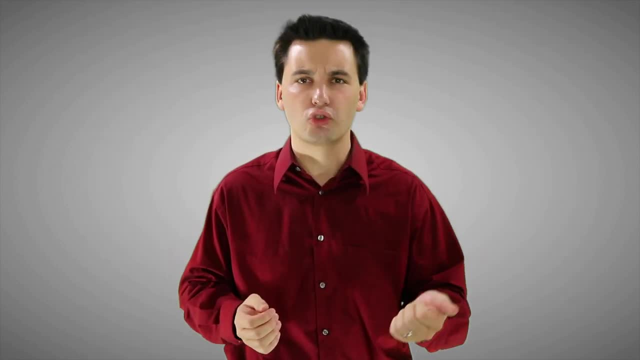 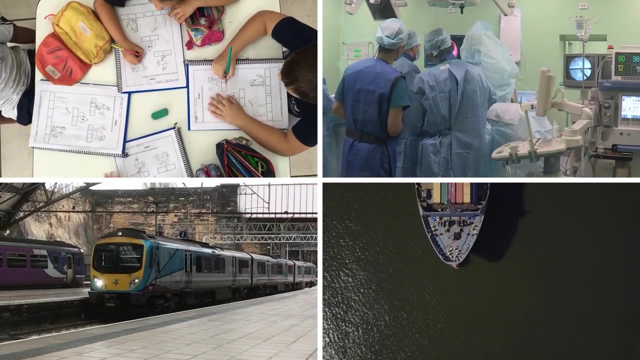 state with more people living in it, who have actually less of an impact on the actual results of the electoral votes for their state. Economically, we could look at how population distribution impacts funding of schools, hospitals and government services. We could also look at how it impacts the amount of goods and services that can be provided by the 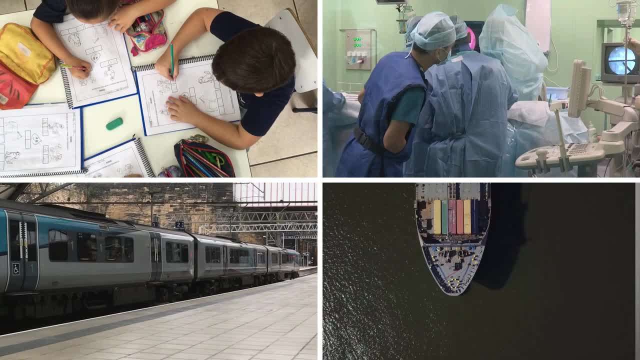 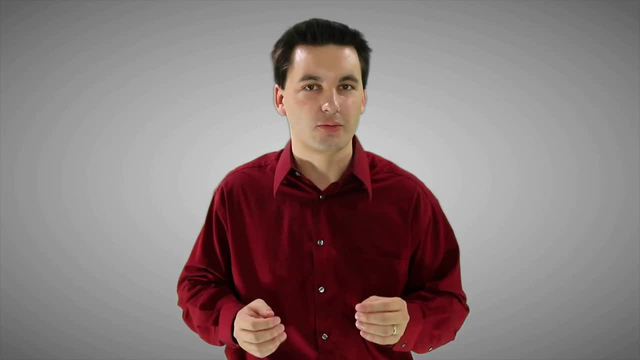 private sector as well. Areas that have more people living in them will be able to gain access to more goods, services, resources and be able to have more access to different types of jobs, compared to areas that have less people living there, where they might actually have to travel farther to. 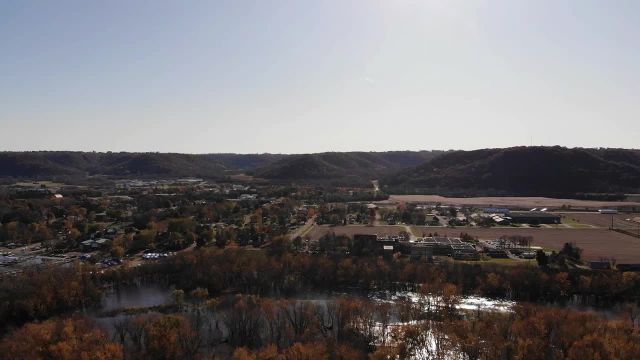 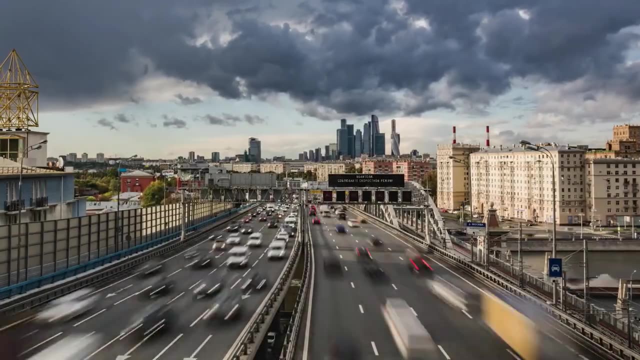 get the same services compared to someone who lives in a more densely populated area. Another economic consequence would be that actually, we start to see this cost of living go up. in more densely populated areas, Taxes are higher, goods are more expensive and even just. getting a house can be harder compared to places that are more sparsely populated, where, we start to see, taxes are lower and the cost of living decreases. Socially, we could look at how population distribution actually changes, even family sizes, Areas that are more sparsely. 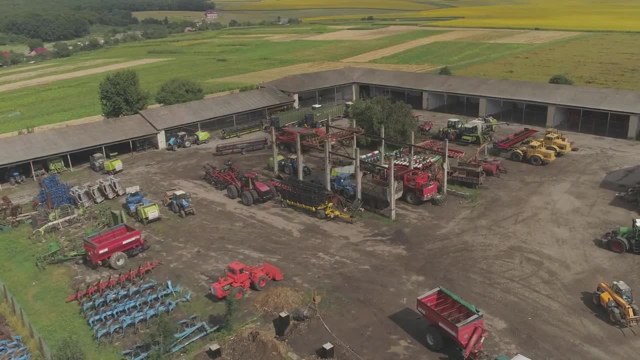 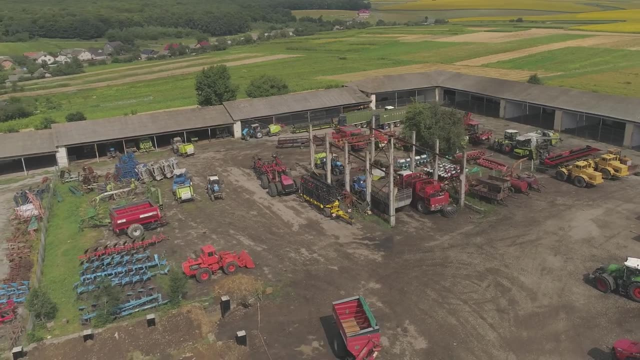 populated, often times are in more rural communities and that tends to have larger family sizes, so people can help out around the house and on the farm and reduce the cost there. However, as we start to move into cities, we start to see that family sizes go down. 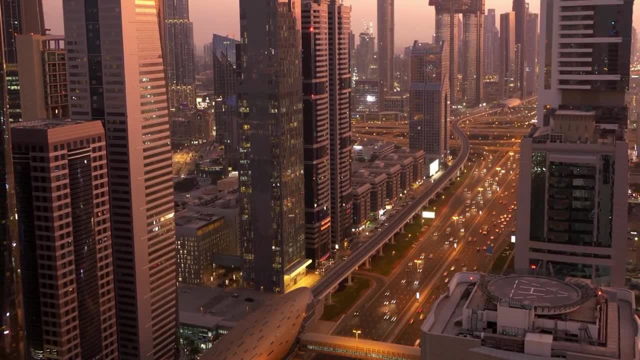 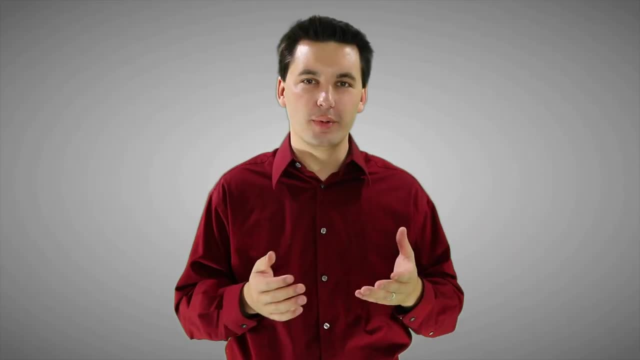 and that's because it's more expensive to have kids in the city and also there's less economic advantages to having kids: It's expensive and you don't have as much room. Or we could even look at health, where we could see that urban areas are going to have more access to better 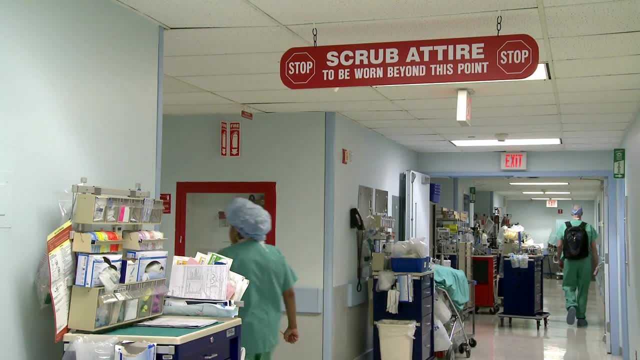 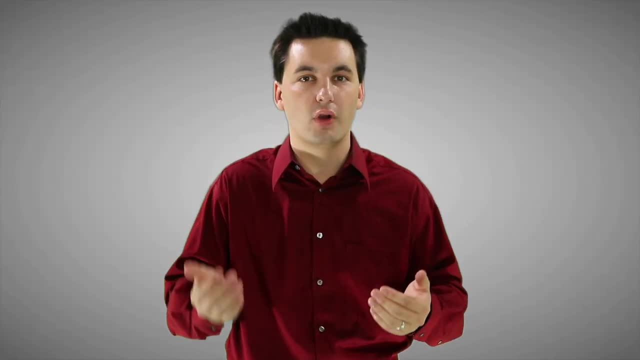 healthcare systems. they're going to have more access to different services that allow them to live healthier lives. On the other hand, though, we could also see densely populated cities that struggle with food deserts and crime rates, where you actually could be put at risk for living. 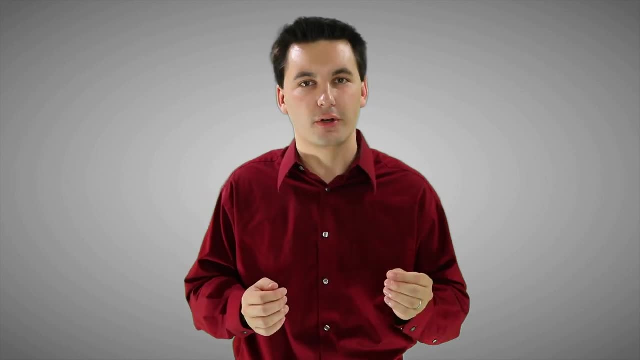 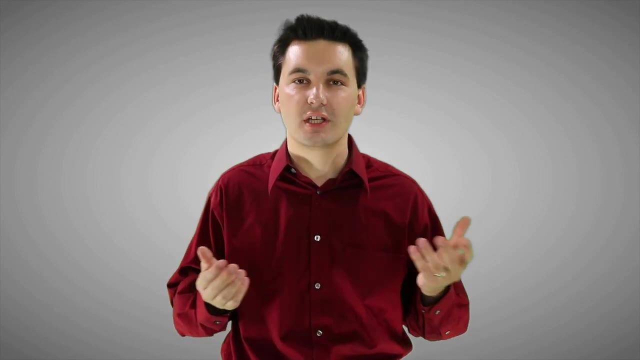 there. If we look at rural communities, they might have to travel farther to be able to get those services. particularly as we get into like specialized medicine, They probably will have to go to larger urban areas to get those services. Lastly, we could talk about the environment. 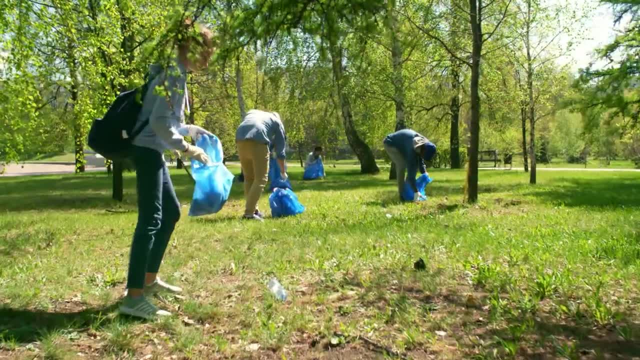 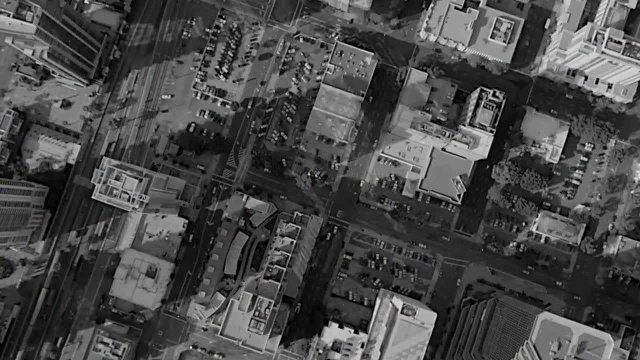 where we could see that areas that actually have a lot of people living in it risk a lot of pollution, and they also risk losing parks and natural green land. So if we look at rural landscape as we start to see cities turned to concrete jungles, this then actually increases. 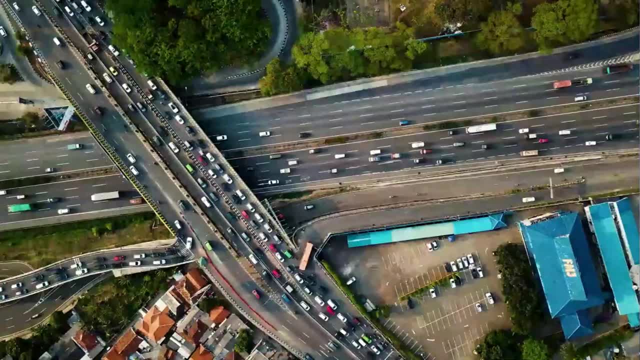 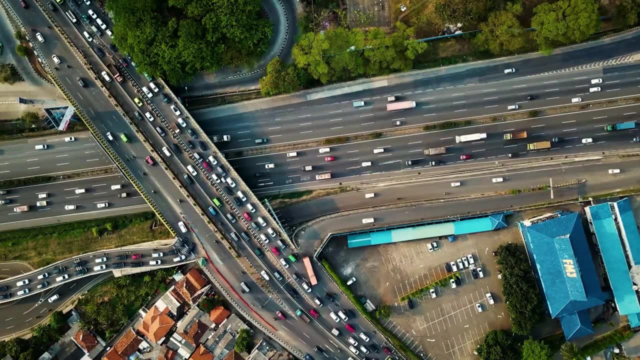 water runoff, which increases water pollution. The more cars that are driving, sitting in traffic, that also adds to air pollution, Not even to talk about the amount of energy needed, which, if it's being powered by a coal power plant, also again increases our air pollution. 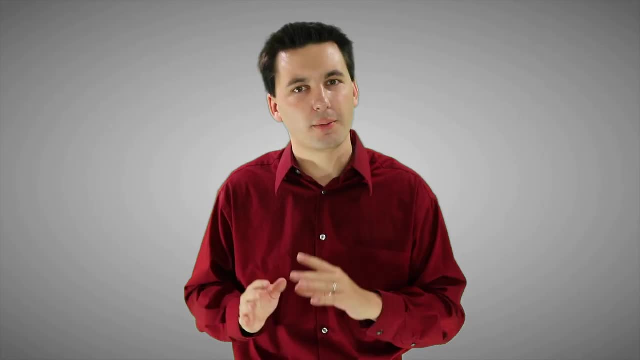 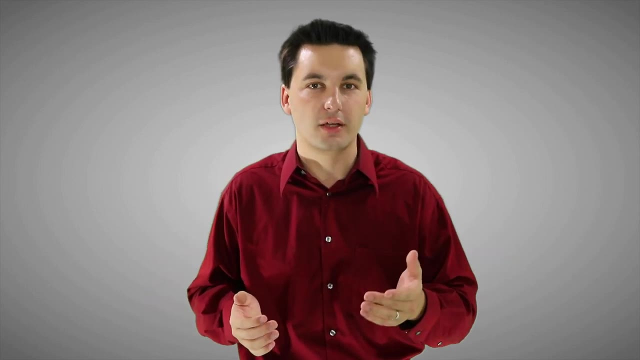 And cities too risk actually urban sprawl. It's a concept we'll talk about more in unit six, but essentially it's the city continuing to grow out, where we might start destroying farmland in our arable land to actually just have people living there, On the other hand. 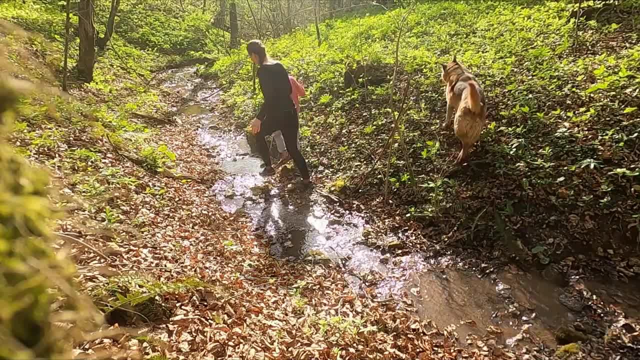 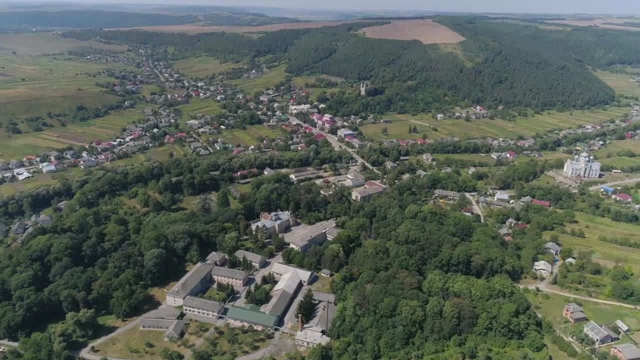 though we could look at how sparsely populated communities have more opportunity for citizens to go outside to enjoy nature, to be able to have their kids play out in the yard. They don't have as many busy streets That causes more air pollution They might have. 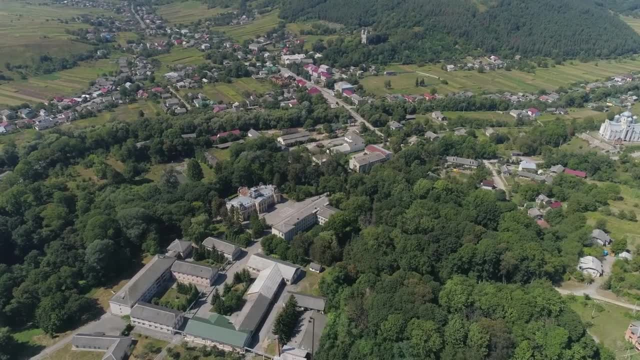 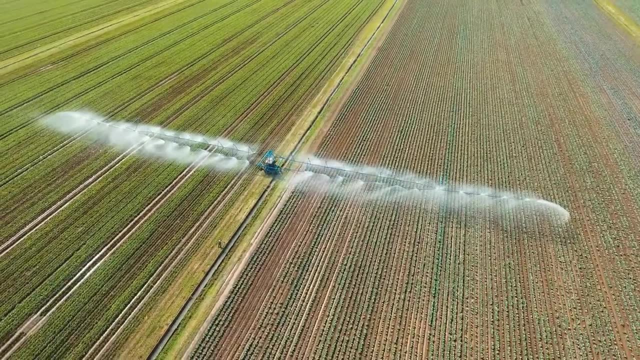 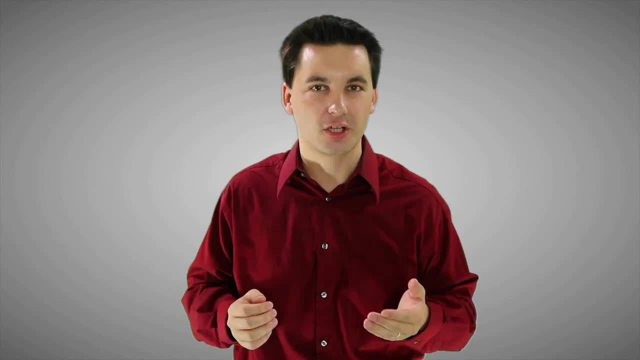 in sparsely populated areas. Now, since we're on the topic of the environment, one thing that all, Now, since we're on the topic of the environment, one thing that all societies have to be aware of, is their carrying capacity. The carrying capacity is simple, It's. 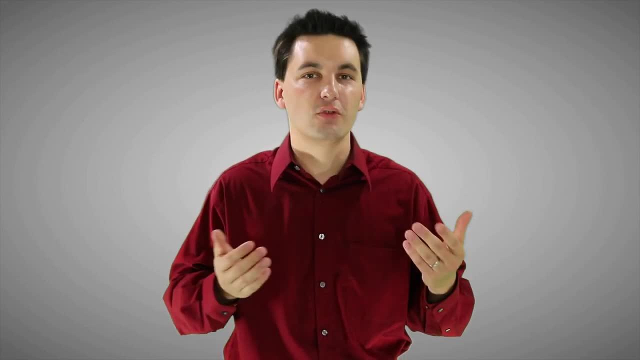 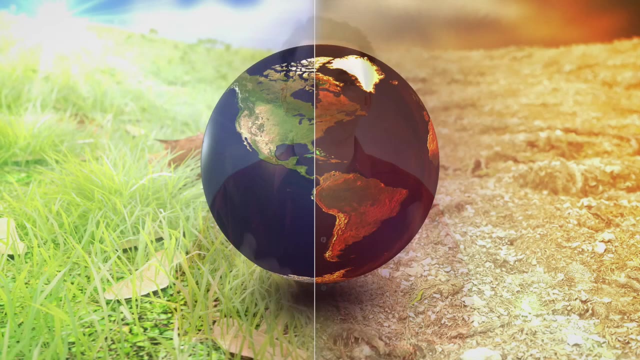 just how much life can be supported by the environment without damaging it. If we start to exceed our carrying capacity, well, we risk damaging the environment. We'll start to see desertification happen, a depletion of the natural resources in the earth, and we're also going to 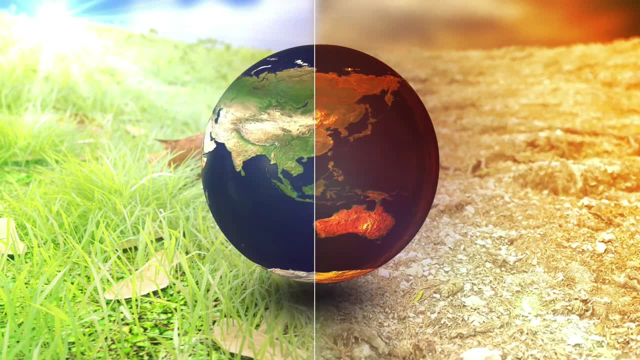 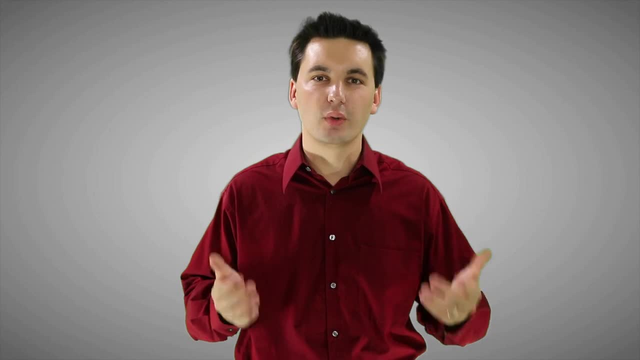 run into overpopulation issues. All of this could be very detrimental for society. Already, we're seeing some parts of the world reach their carrying capacity or start to get close to it, and this can be really dangerous. This can lead to hunger, it can lead to water shortages, it can 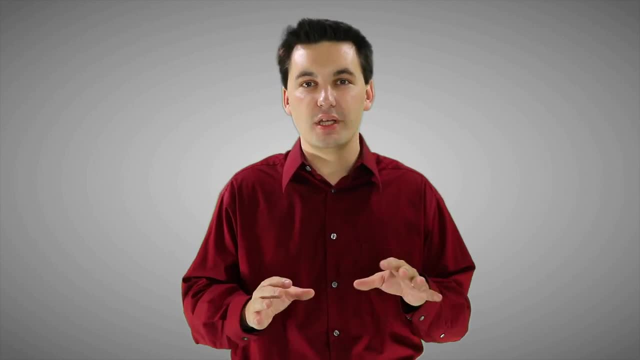 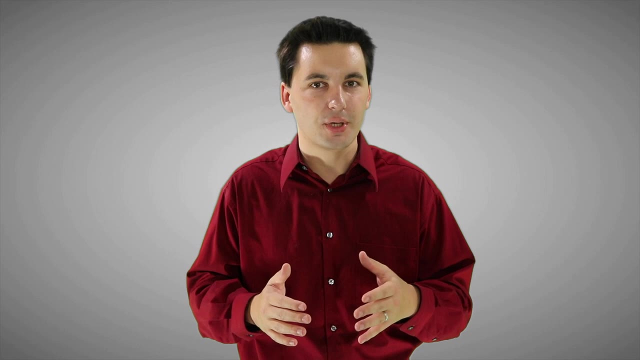 lead to an increase in crime and refugees and, in extreme cases, even terrorism, as people become desperate to survive, And this impacts not just the region that it's happening in, but the rest of the world. Now it's definitely not all doom and gloom here. There's a lot that can be done to. 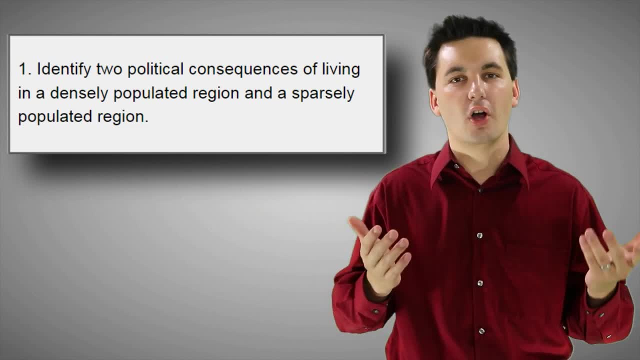 be able to help societies that are already struggling with overpopulation, and there's also a lot that countries can do to protect themselves. So, if we're going to be able to prevent it from occurring- But we're going to talk about that later in Unit 2.. Now what you 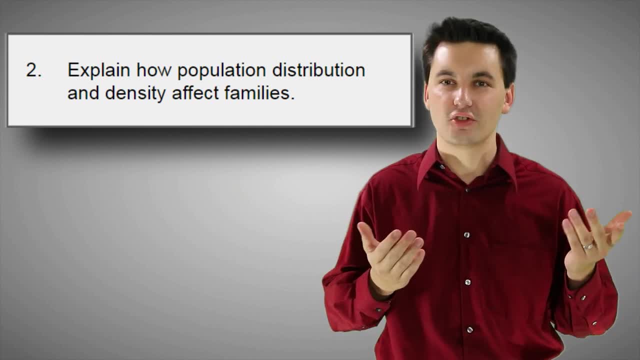 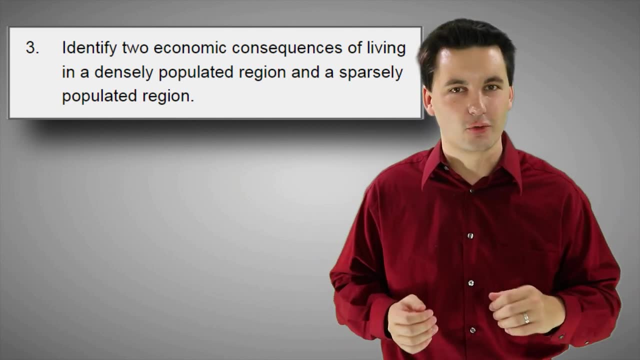 need to do is practice all these concepts that we just talked about. You can see the quiz questions on the screen right now. Make sure you answer them and then again check your answers in the comments below. Also, thank you so much to everyone who's been subscribing The support. 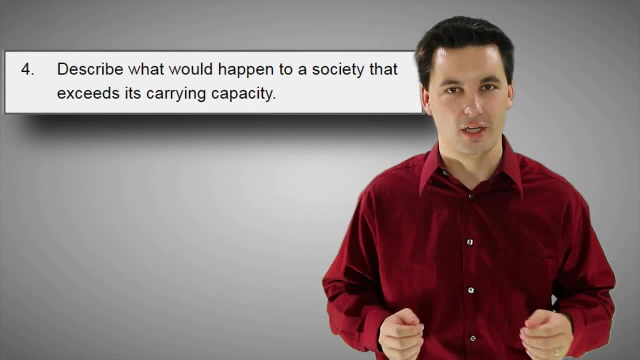 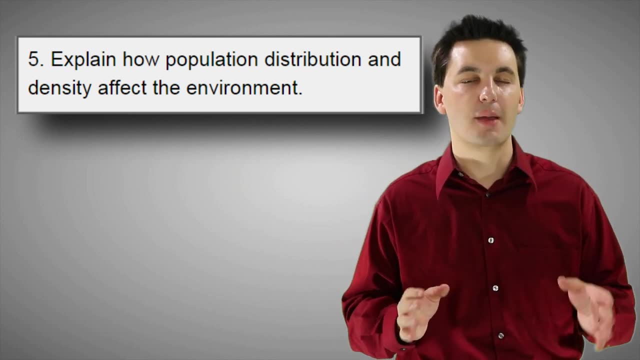 has been overwhelming. I'm so glad you guys are finding value in these videos. By subscribing, you're allowing me to keep making more videos for you guys, and I'm just happy that they're helping you out. All right, that's all the stuff we have for today. Make sure you check back next. 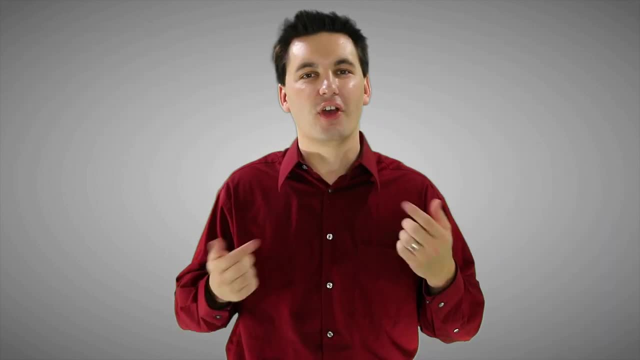 time when we'll go into 2.0., 2.3.. Until then, though, geographers, I'm Mr Sin, and well, I'll see you online.